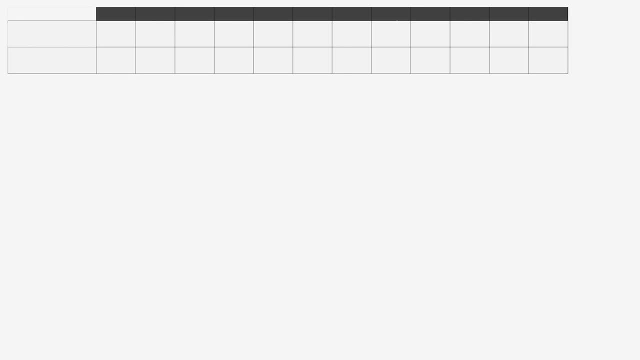 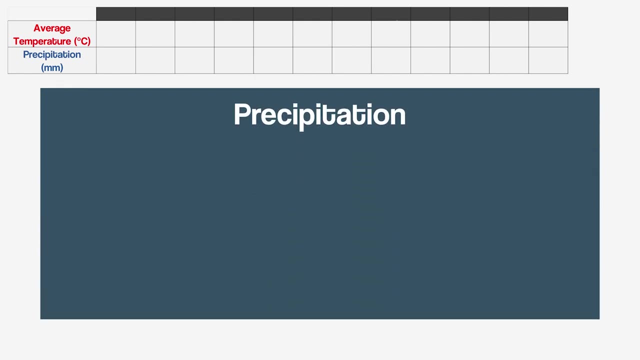 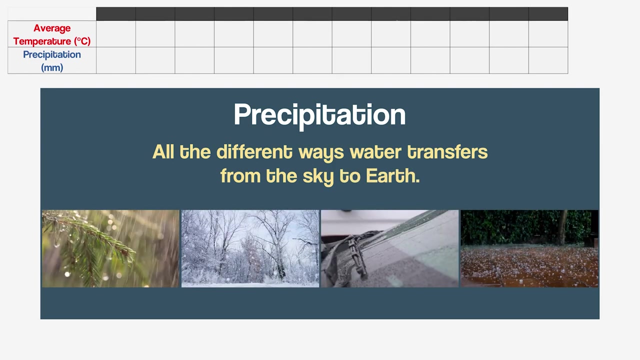 place. Most basic climate graphs show two things: Temperature and precipitation. If you're not familiar with the word precipitation, it just means all the different ways water transfers from the sky to earth. So rain, snow, sleet, hail- all of that added together. 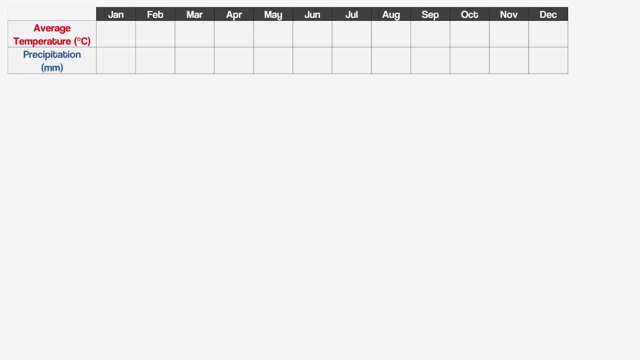 Then we just have the months of the year across the top of the table, So we can easily see that in January the average temperature is 4.8 degrees celsius and 59 millimetres per hour. The average temperature is 4.8 degrees celsius and 59 millimetres per hour. 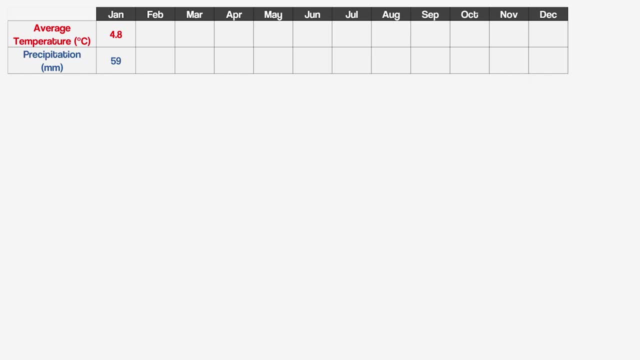 February is a little warmer, with an average of 4.9 degrees celsius, and it's a bit drier, with an average of 50 mil of precipitation, and so on. We'll start this graph off by drawing the x-axis which will show the months of the year. So we're going to need 12 spaces for that. You'll find. 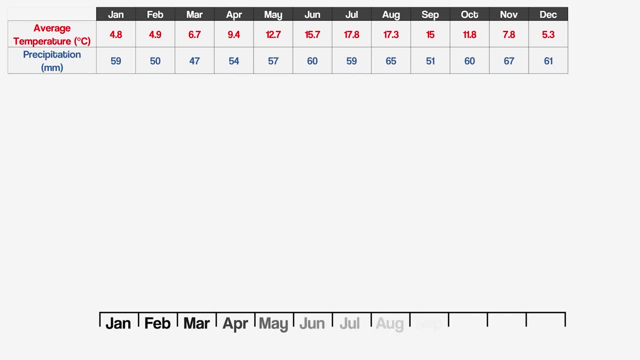 that some climate graphs label the x-axis with a shortened version of each month. Some use numbers, so month 01 is january, 02 is february, 03 is march and so on, But most climate graphs simply use the first letter of each month. Let's make sure the x-axis is labeled too. Next up, we'll add: 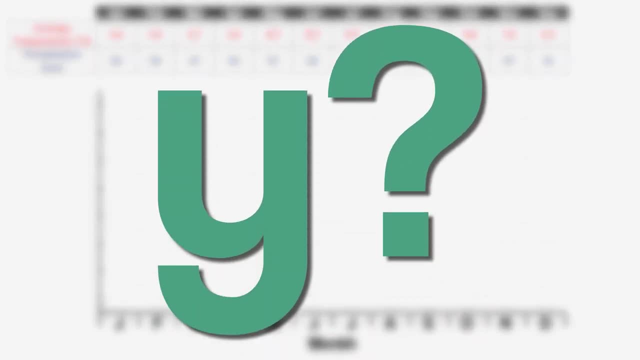 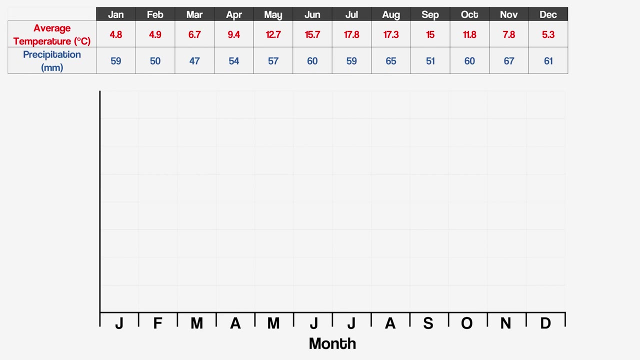 a y-axis. Why? Because we want to. We're going to plot the temperature against the axis. The highest number we have in our data is 17.8 degrees celsius, so I think we're going to want to add a y-axis. So I think the numbers on this axis should go up in fives, up to 20.. And again, 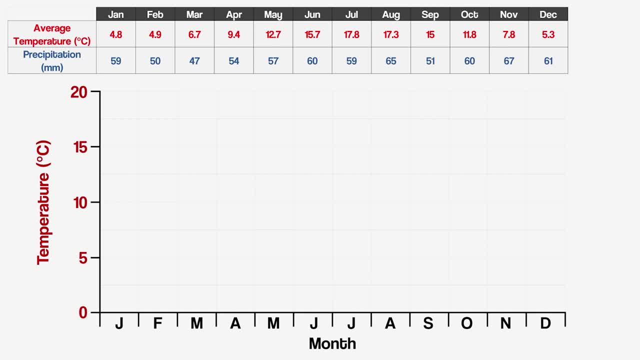 it's always good to make sure the axis is labeled. Climate graphs have a second y-axis. This is the one that we're going to use to show precipitation. It looks like the largest number we have here is 67 mil, so I think this y-axis can go up to 80,, 10 at a time And, yep. better label it At this point. 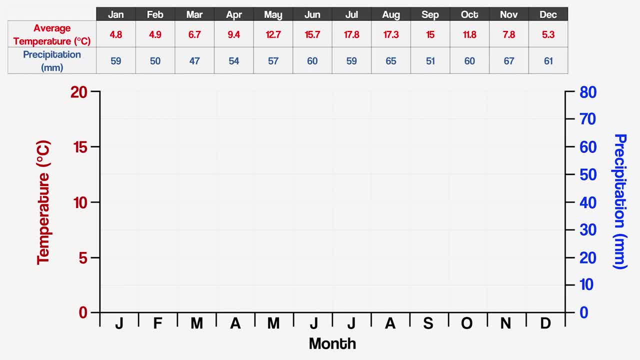 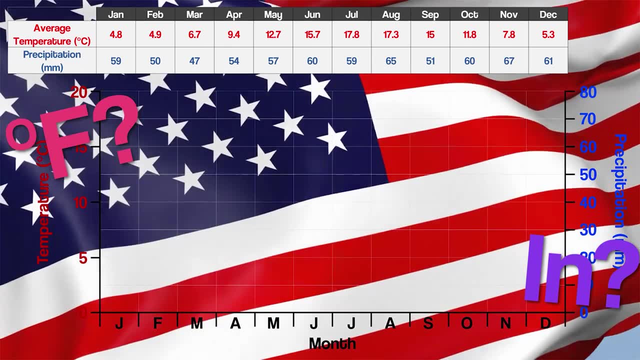 we should probably tell you that you might also see climate graphs with a lower temperature than those that show temperature in Fahrenheit and precipitation in inches. Yes, America, we're talking to you. We're not saying that one unit is better than the other. 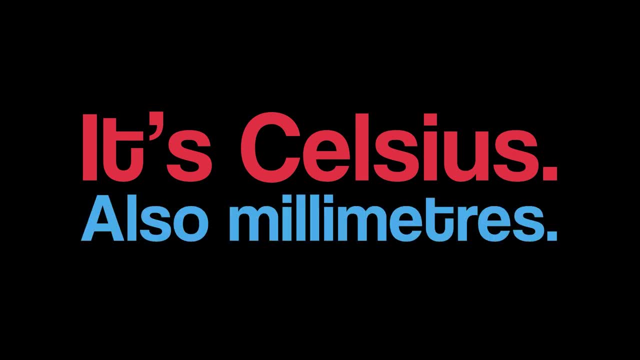 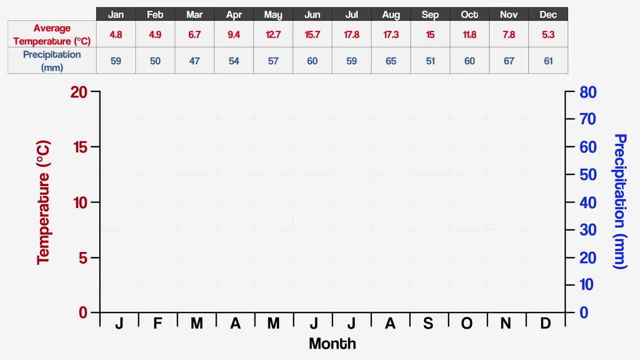 Oh wait, yes, we are. Celsius is better. Stop being weird and use Celsius already. America, It's time we put our data on this graph, starting with precipitation. This is always shown using the y-axis. The bars are often- though not always- blue, So January had 59 millimeters of. 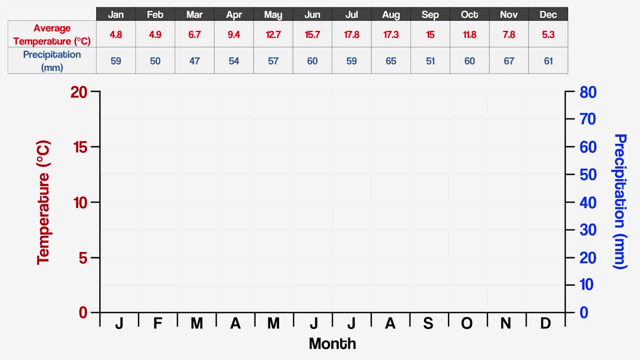 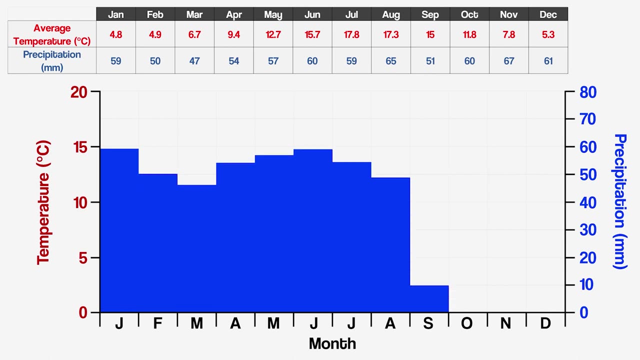 precipitation, And we need that to match the correct y-axis. So that has to match up to here. And then we add our bar February is 50 mil, which is here, And we add another bar, March is 47 mil, and so on all the way to the end of the year. Now for the temperature. Temperature is plotted as a 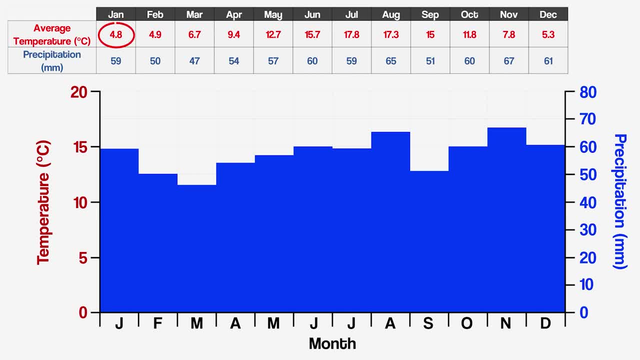 usually in red. January averages 4.8 degrees Celsius. Just like before, it's important to make sure we line it up with the correct y-axis. Then we put a little dot or a cross in the middle of the January section. Then we do the same for February, which is 4.9.. March, which is 6.7.. 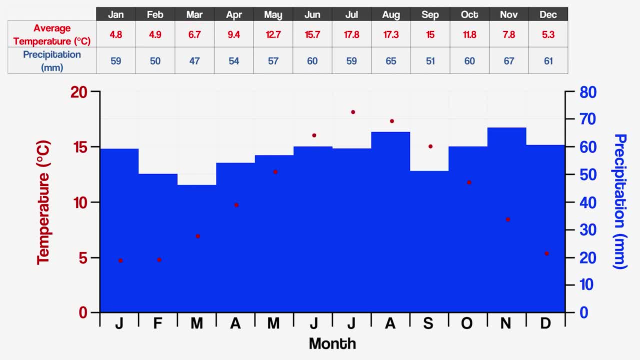 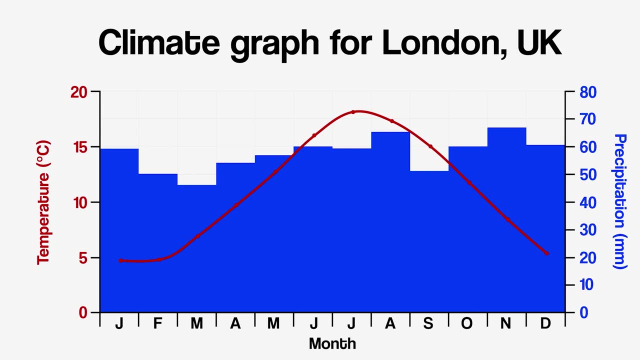 And for the rest of the months of the year. Now that's done. we'll just join it all up with a curved line. That's really satisfying to watch. And there we are, One climate graph. Actually, yeah, this is just one climate graph, And other ones can look very. 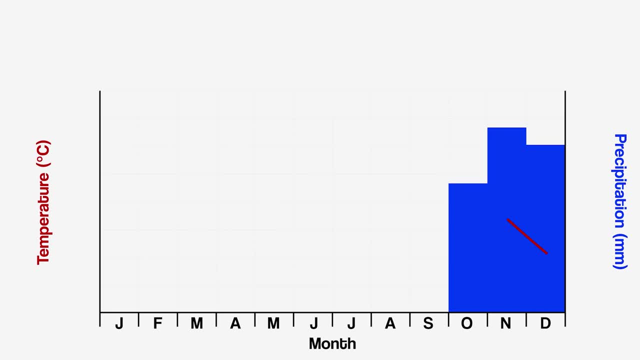 different to this. We're going to need to make some changes to our y-axis. to show you what we mean, Firstly, we're going to change our temperature axis so it starts at minus 70 Celsius all the way up to 50 Celsius. You can do that on a climate graph, Don't worry. Oh, let's also add a. 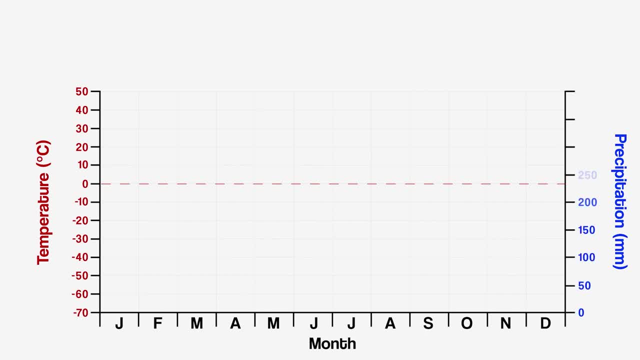 temperature scale. On the other side, our precipitation scale is going to need to go all the way up to 400 mil. Yep. things are about to get wild, So we'll start by putting London back on here. Remember, this is the same information as before. It's just been squashed up a lot to match the new scales we put. 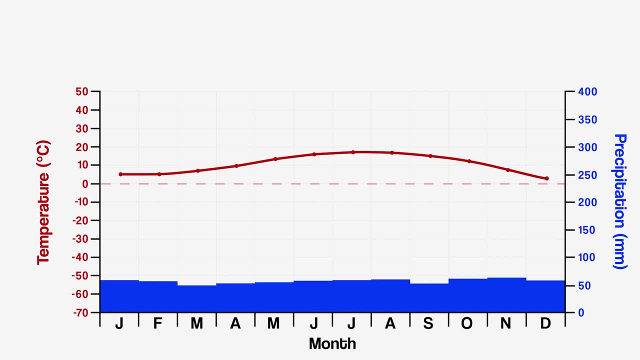 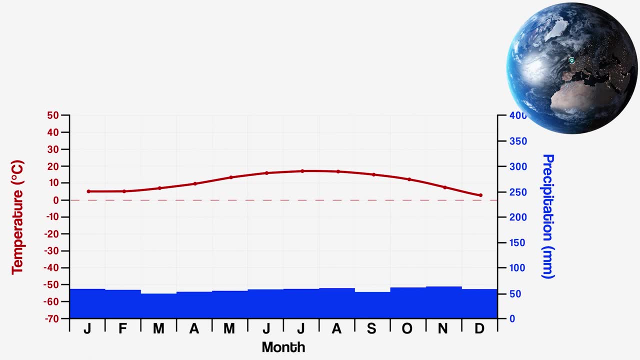 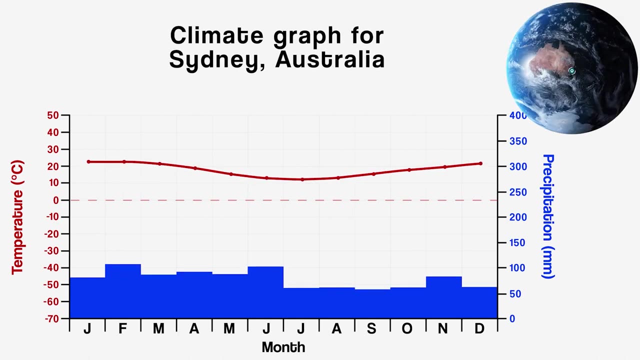 on our y-axis, But where shall we show next on our climate graph? Ah, I know London is in the northern hemisphere, so the warmer months are around June, July and August. If we were to choose somewhere in the southern hemisphere like Sydney in Australia, their seasons are the other way around.